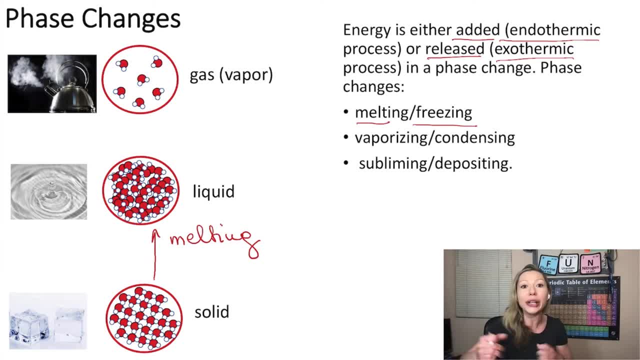 molecules can gain this mobility to pass each other. So melting is going to be an endothermic process. when energy is needed to be added, What happens during freezing? Well, during freezing, we are going to actually release energy, which is going to be an exothermic process because from 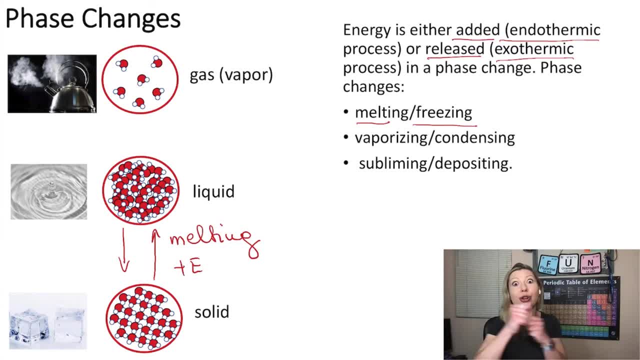 the passing state. the molecules pass each other. They are just going to be stopped in one spot and kind of vibrate. okay, So this is going to be freezing And energy is going to be released in this case. Okay, now what? 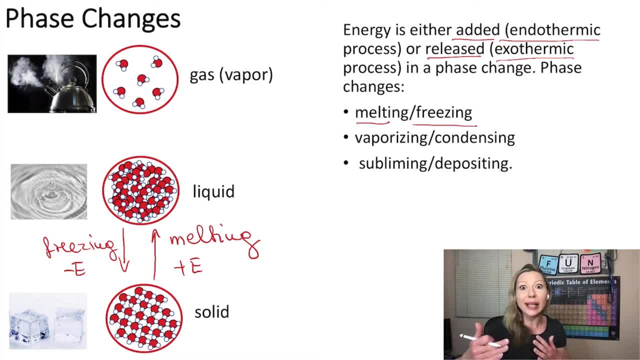 happens when we go from a liquid to a gaseous state. We are going to have vaporization right. Liquid to a gaseous state. As I said, in liquid we are passing each other with the molecules. in the gas, Molecules are just zooming, So this is going to be an exothermic process. When we go from a 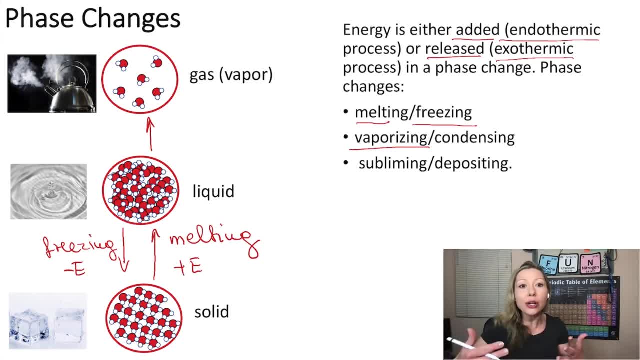 zooming, zooming around. So we need to add energy to get to the gaseous phase. So vaporization is going to be an endothermic process. Now what happens when we have condensation? In that case we are going from a gaseous to the liquid phase, And because molecules are going to be closer to 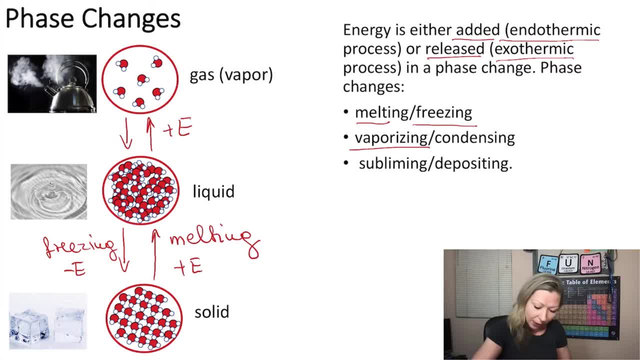 each other. we are going to have an exothermic process when energy is actually released. Now we also have to talk about sublimation and deposition. So the process of subliming is simply going from the solid to the gaseous phase right away. So this is why, for example, dry ice is called. 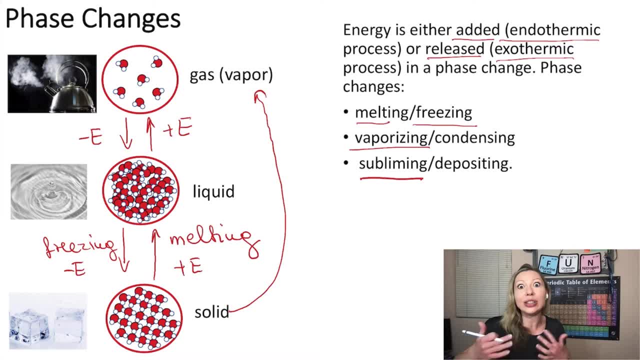 dry ice. Solid carbon dioxide is dry ice. You will never see it in a liquid phase at a 1 atm pressure, because at atmospheric pressure it simply sublimes, goes from the solid to the gaseous phase. That's from where the name is coming from: dry ice. 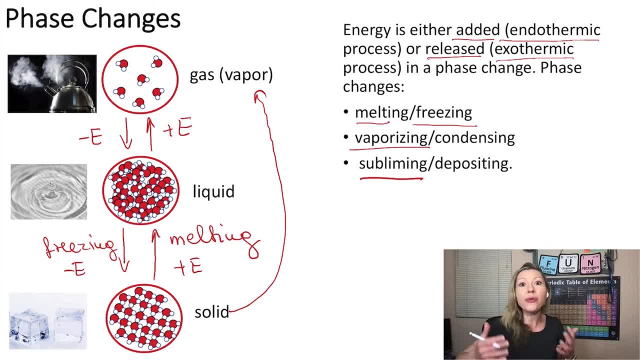 because you will never see the liquid. Okay now, if we have to go from a solid to a gaseous phase, where molecules are zooming around, do you need to add energy or will you release energy? Well, in that case, we need to add energy, right? So sublimation is going to be an endothermic process. 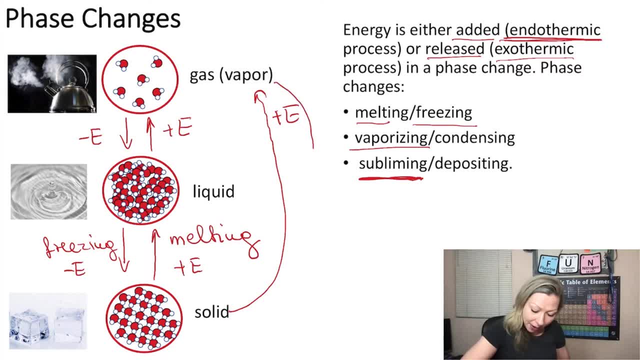 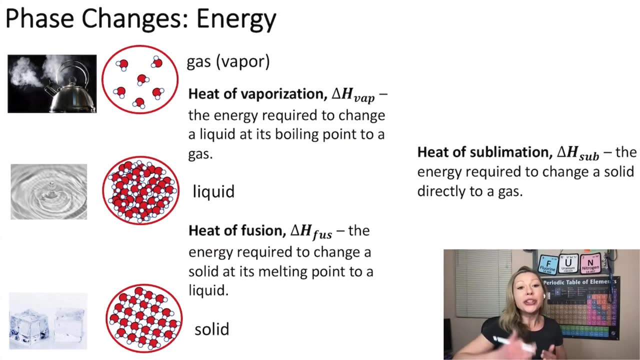 We are depositing. so, going from the gaseous phase back to the solid phase, we are going to release energy, So this is going to be an exothermic process. Okay, I hope this makes sense. Let's talk a little bit more about the energy changes. So when we are actually going from a solid to a 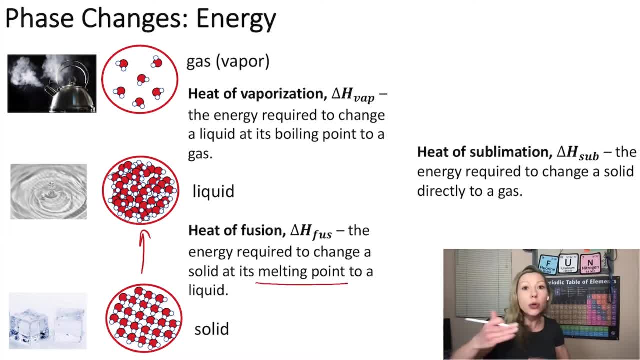 liquid phase at the melting point, we are going to call the energy change associated with the process, the heat of fusion, delta H fusion. And when we are going from the liquid to the gaseous phase at the boiling point, we are going to call the energy required for this change. 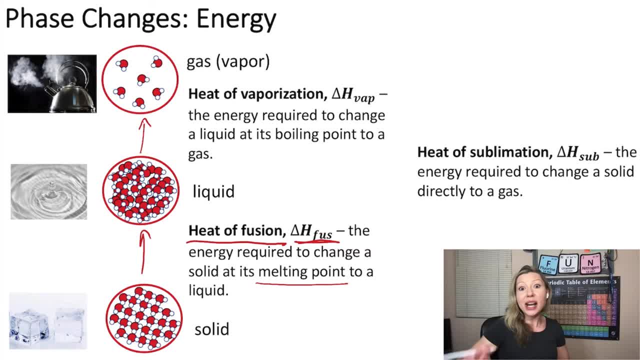 the heat of vaporization And we are going to have the heat of sublimation, which is simply the energy required to change from a solid directly into a liquid. So we are going to have the heat of fusion directly into the gaseous phase. Okay, so we know that we need to add energy. 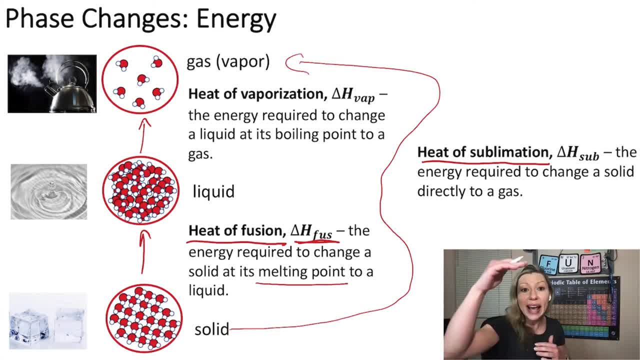 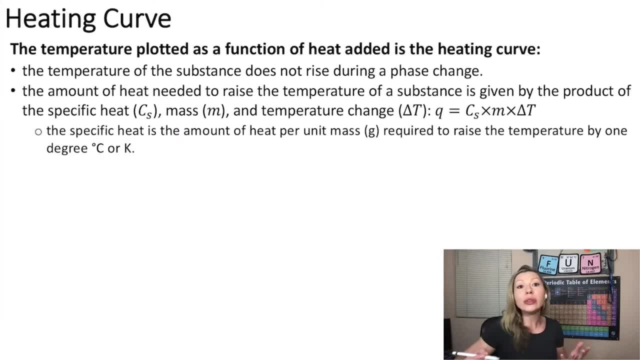 to go from a solid to a liquid, from a liquid to a gas state or from a solid to the gaseous state right away. Now let's talk more about this using the example of a heating curve. The heating curve is simply the temperature, plotted as a function of heat added to a substance. So let me draw this. 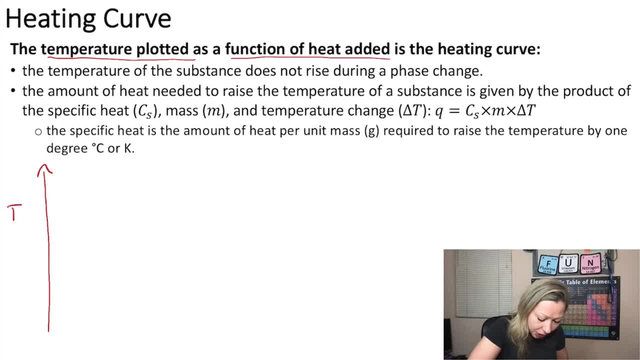 to you. Here I'm going to have the temperature, let's say degrees Celsius, And here I'm going to have the heat added. heat added. Now, if I start, let's say here, let's say this is minus 25 degrees of Celsius, As I add heat to water, for example. 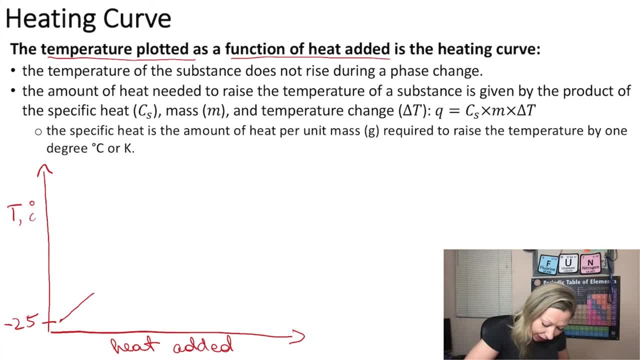 then my temperature will rise, And the temperature will rise up to the melting point. At what temperature does water melt? at 180 M pressure, At zero degrees Celsius. right, So I can achieve zero degrees Celsius here And now. I'm going to have the process of melting, So notice. 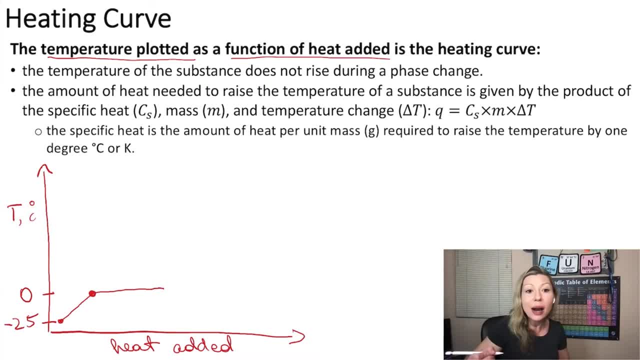 that when I'm melting, actually the temperature of the substance does not rise. Okay, so during the phase change, the temperature of a substance is always going to be constant because the energy is used to actually separate the molecules from a solid phase to a liquid phase. Okay, so the 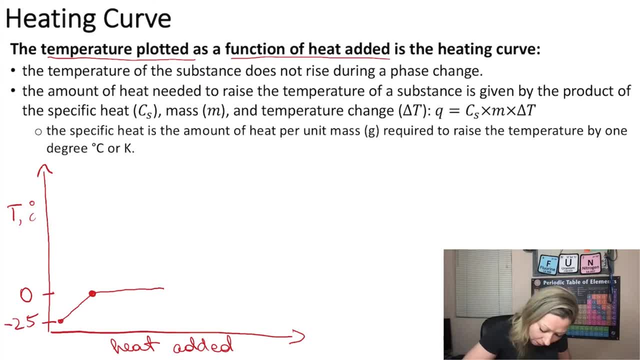 energy is used for the phase change. Now, once I changed all my solid into a liquid, so I melted all of it, then I can increase again the temperature, and I can do it up to 100 degrees Celsius, right? So let's take a look at different parts. So let's call this part A to B, C, D, E and F. 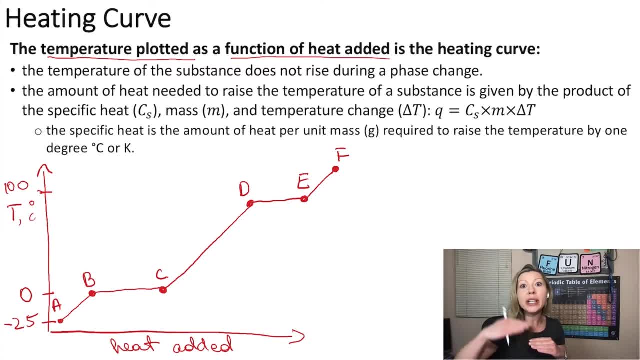 When I'm going from A to B, I'm going to have the temperature rise up to 100 degrees Celsius. When I'm going from A to B, I'm simply increasing the temperature from minus 25 degrees Celsius to zero Celsius. Okay, so here I'm going to have a solid or ice, if I am talking about water. 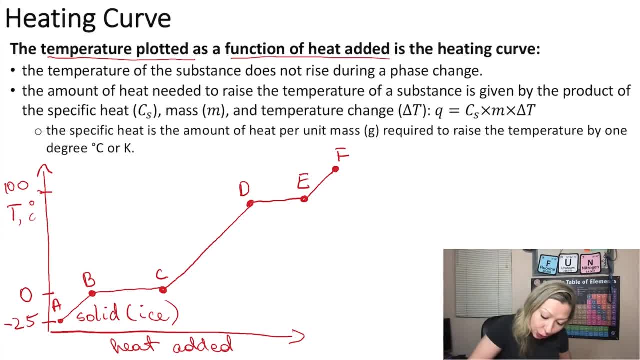 and the amount of heat added to raise the temperature of a substance is going to be given by the product of the specific heat multiplied by the mass and the temperature. so the delta T, And just a reminder that the specific heat is the amount of heat per unit of 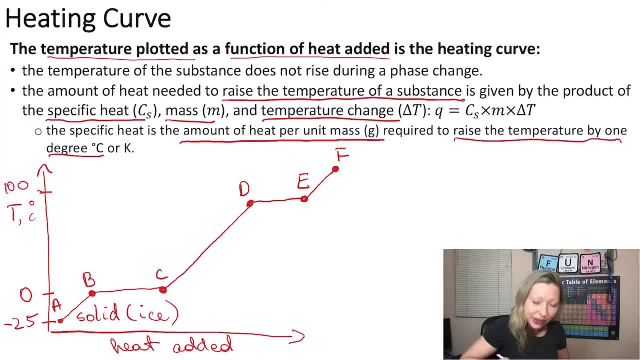 mass required to raise the temperature by one degree Celsius or Kelvin. Okay, so this is how I can calculate. how much heat do I need to add to actually increase the temperature of a solid or, in this case, ice? Now what happens when I am in the part where I have B to C, So you can see. 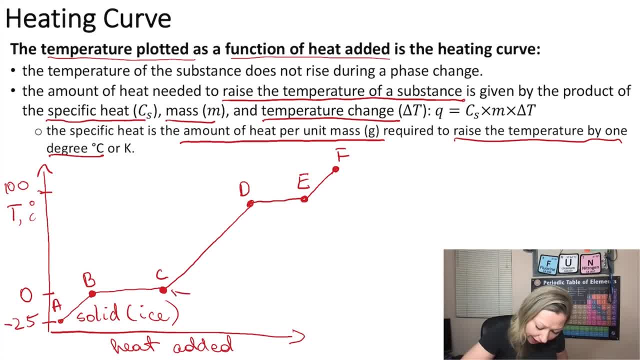 from B to C, the temperature doesn't change. Here I have zero degrees Celsius, and this is the process which is called melting. So during this process, I can calculate the temperature added using the heat of fusion. Okay, so delta H fusion. This is usually given by energy per mole. 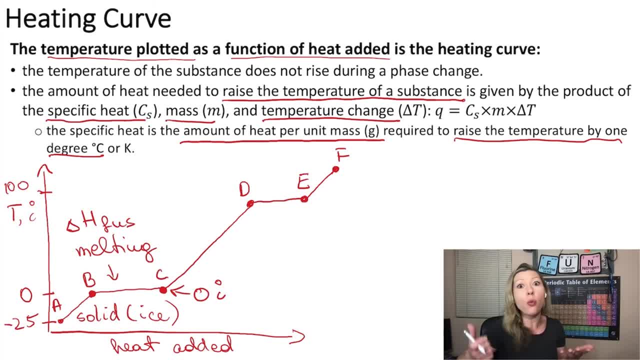 So let's say that the heat of fusion of water is- I'm just giving you a number- 10 kilojoules per mole. Then if I need to melt one mole of water, I need to add 10 kilojoules of energy If I need to melt two moles of water. 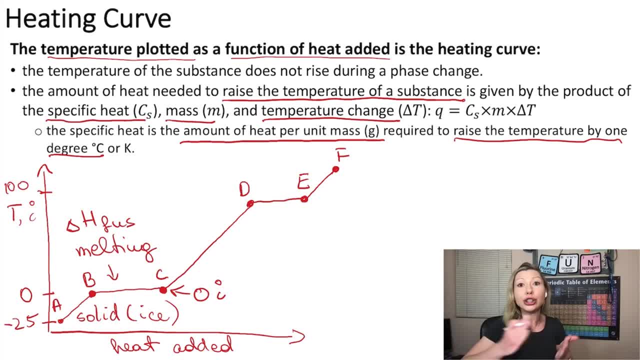 then I need to add 20 kilojoules of energy, because two times 10 kilojoule per mole. I hope this makes sense. Then what happens when I go from point C to D? In this case, I'm going to. 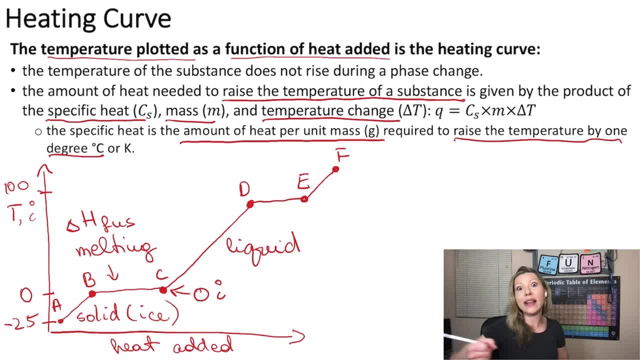 have a liquid right, Let's say liquid water, And again I can calculate the amount of heat added if I know the specific heat, the mass and the temperature change right Now. also notice that this line here has a smaller slope than this line here. This simply means that I need to add. 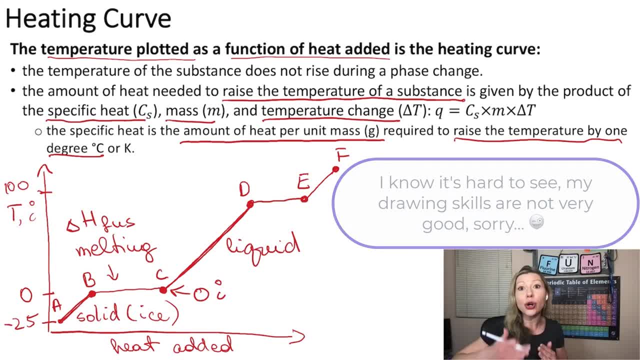 more heat to change the temperature of water. Now, when I get to 100 degrees Celsius right here, my temperature is constant. This means that I have a process called vaporization, Vaporization, Vaporization, Vaporization, Vaporization.